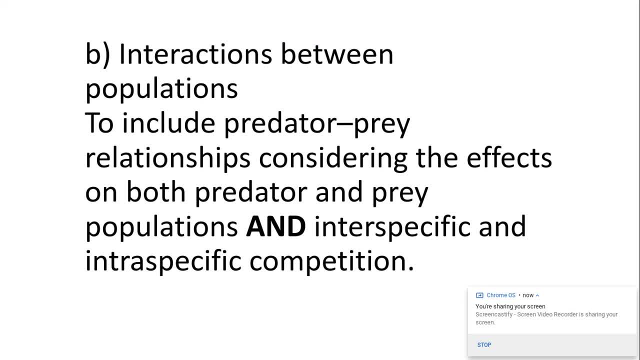 Welcome biologists. Today we are going to be looking at 6.3.2, taken from Populations and Sustainability for A-Level Biology, A OCR. We're looking at B, Interactions Between Populations. And again, this is a very general knowledge, quite an easy lesson objective to get your head around. really, We're looking at predator-prey interactions and intraspecific and interspecific competition. Now, we've looked at that before, we've mentioned it before, so it's nothing really drastically new. 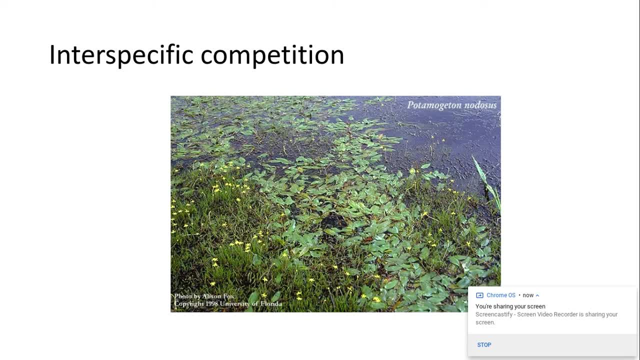 So interspecific competition. this is between two different species. So here you can see a plant on the top of the water there and that'll be blocking out the sunshine, so therefore the plants underneath cannot get the light. So that's interspecific competition, competition between light for different plants within the water. 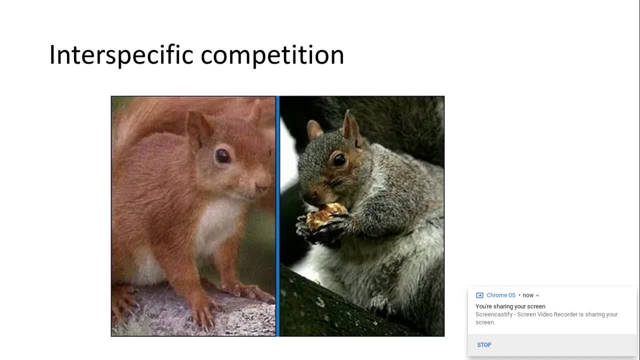 We also have another example here between the grey and the red squirrel In interspecific competition, different species competing against each other. Now this one's for food resources. so the grey squirrel has done really, really well and it's out-competed our native red squirrel, which isn't the best, but hey-ho. 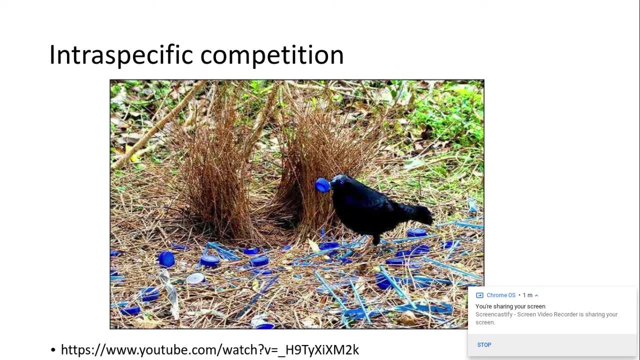 So intraspecific competition. sorry, this is an example of where we have competition between members of the same species here. Now, the example that I've given here. this is the bowerbird. There's a great video there to watch if you want to. 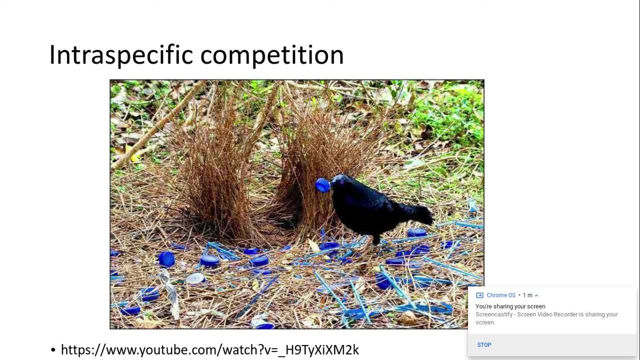 And a bowerbird will compete with other bowerbirds to win- Win over the females, and in this case it will do it via creating a really vibrant bower in order to attract the female. And I'm sure you can think of lots of intraspecific competition between members of the same species. members of the same species. 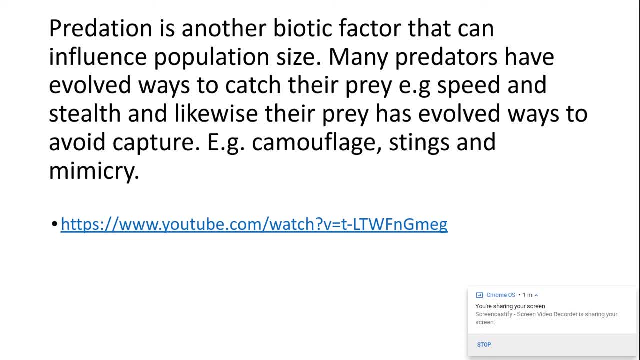 Predation. this is a biotic factor we mentioned before which can influence population size. Many predators have evolved ways to catch their prey, for example speed and stealth, like in a cheetah, And likewise their prey has avoided ways to get captured. so, for example, we get the white snow hare for camouflage. 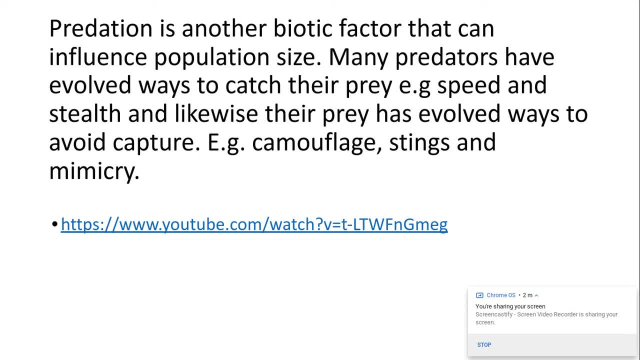 We have stings on things like a stingray and a scorpion, for example, And mimicry. there's a great video if you want to search for that: the mimicry of a mimic octopus. It's fantastic. it can. it's designed to, it's evolved to be, to be, it's behaviour to mimic things like a snake, for example. 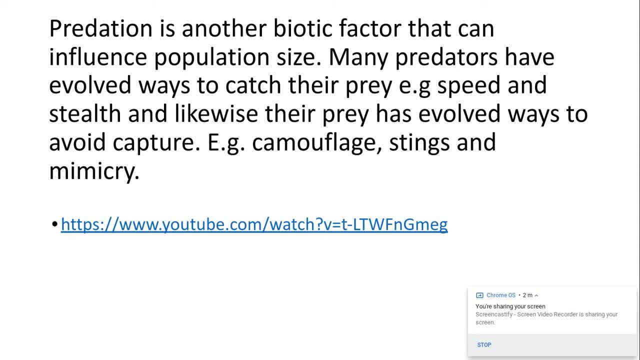 It's evolved to be to be its behaviour to mimic things like a snake, for example. It's evolved to be, to be its behaviour to mimic things like a snake, for example, And fish, for example. it's quite interesting. 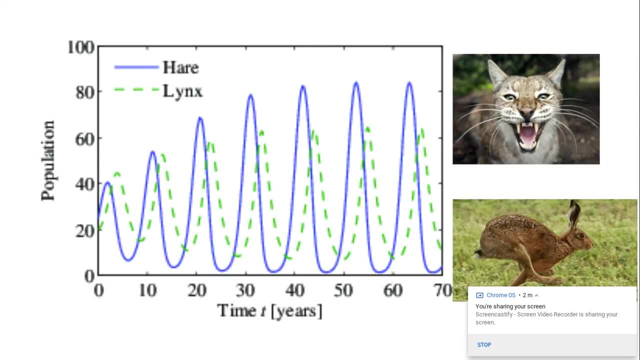 So this is an example of a predator-prey graph. Again this: I think this is really self-explanatory. So as, for example, the hare population increases, which is the blue line, As the hare population increases in size, obviously you'll have more food for the lynx. 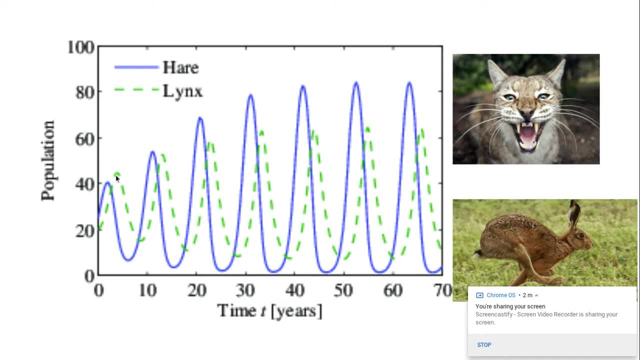 So therefore the lynx population will also increase because it's got more food to eat. But as the lynx population increases, the hare population will therefore begin to decrease, because it's being eaten by the lynx And it's being predated on. 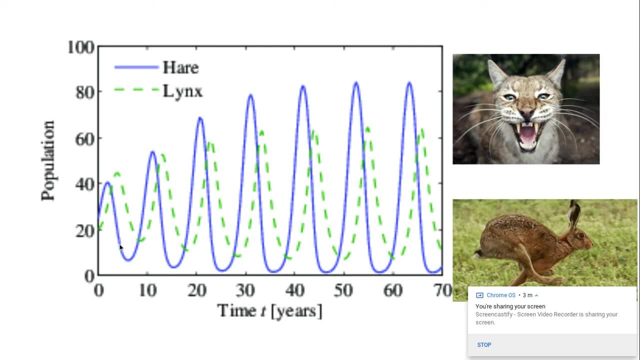 And because the hare population is decreasing, so the birth rate is less than the death rate. because the population size is decreasing, the lynx has less food to eat, So therefore the lynx population will be decreasing again because the birth rate is less. 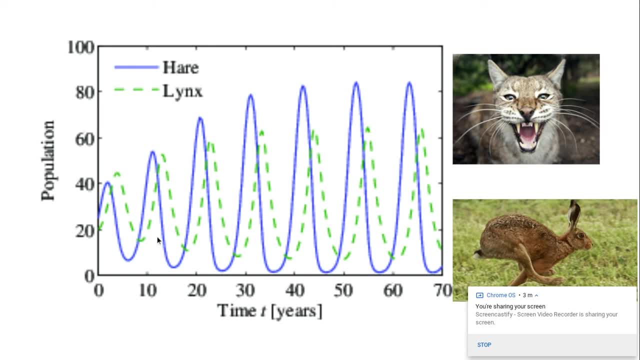 than the death rate And it fluctuates. So predator-prey interactions, population graphs, they fluctuate. All to do with the availability of the food for the predator and over-predation by the predator as well, or predation by the predator. 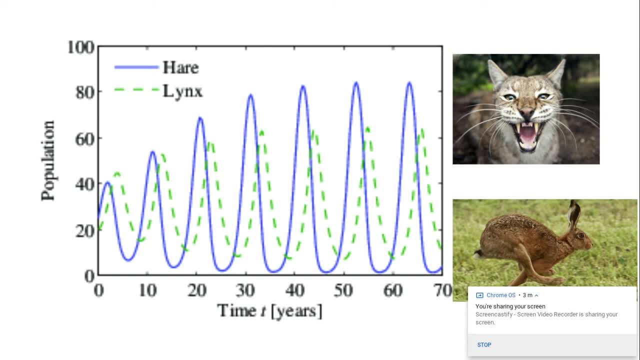 Quite easy, I think, to understand and get your head around this. Don't forget to talk about birth rates and death rates, which one is higher? As the population is rising, the birth rate will be higher than the death rate. But as the population is decreasing, the death rate will be higher than the birth rate. 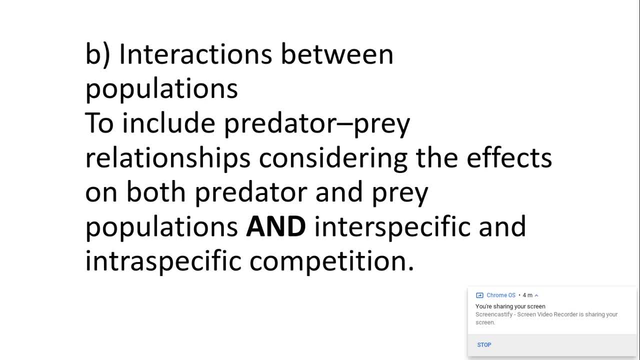 So that's about all you need to know about the interactions between populations. to do with the predator-prey relationships, We've looked at interspecific and intraspecific competition. You just need to be able to identify that from a question and it could give you an. 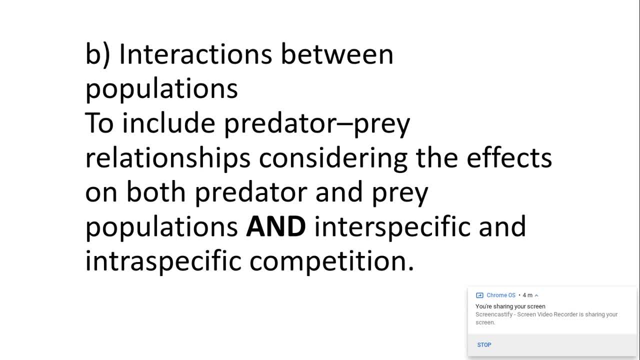 example of any kind of competition that you need to be able to identify as inter or intraspecific competition. So, guys, good luck with your exams. Don't forget to use, do not use the words it, amount, they or size. 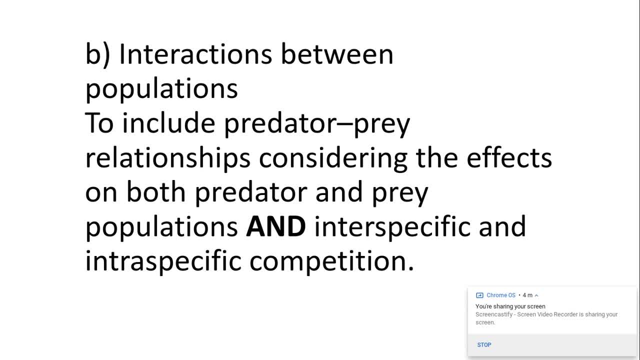 Use good scientific biological terminology. that's going to get you more marks in your exams And good luck.